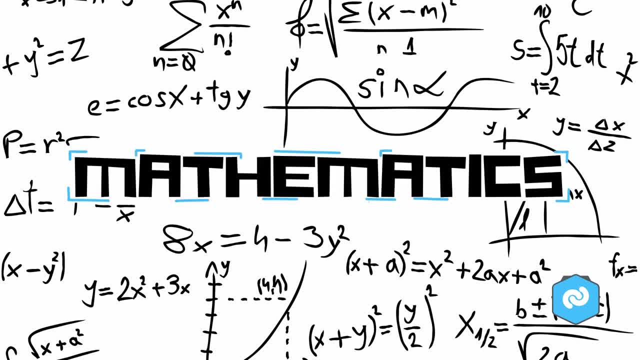 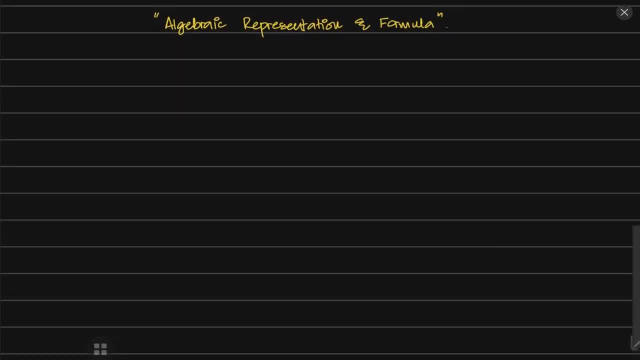 Okay, so we'll start off with algebraic representation and formula today. Okay now, the first thing that you guys need to understand or know over here is what a variable is, what a coefficient is and what your constants are. All right, so let's suppose I have 3x plus 5.. Okay now. 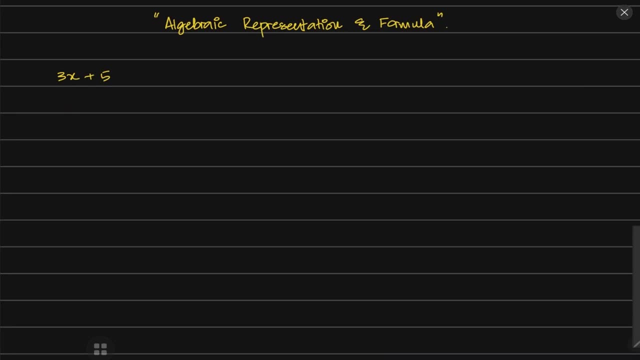 from this guy over here. I'm sure you guys can identify that 3x is going to be the coefficient of x. Okay, this is the coefficient. This x- right here- is a variable. All right, why do we call this a variable? Because it doesn't have a fixed value, The value of this guy. 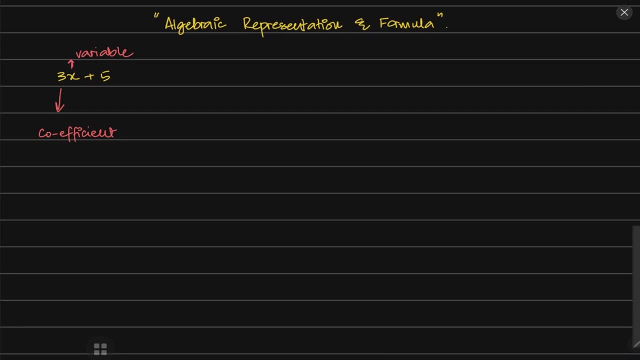 can change at any time. Okay, and the other. on the other hand, we're left with 5, this guy. This is called a constant. All right, why is it called a constant? Because it's a constant number and the value is fixed. It does not change. Okay, now, within this, 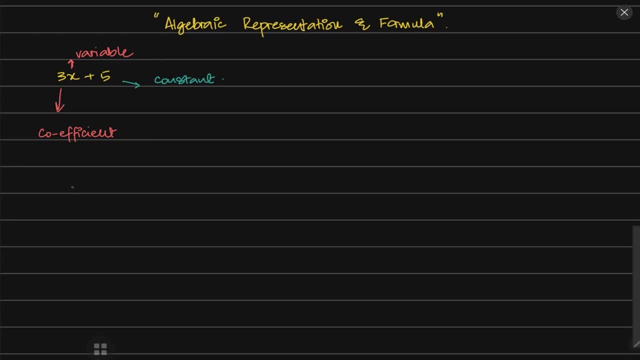 you'll understand, you'll observe. Let's suppose, if I write this down like this, I have 3a squared plus 5a plus 9, let's say right Now, if I write this down individually, what do you? 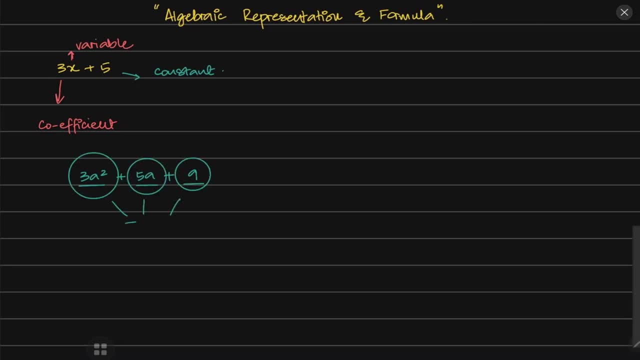 call them. We need to understand that these are terms. Now let's talk about expressions and equations. So, expression, equation- no difference whatsoever. The only thing different about expressions and equations are that expressions are just like this, right here. Okay, They're just a combination of different terms. All right. 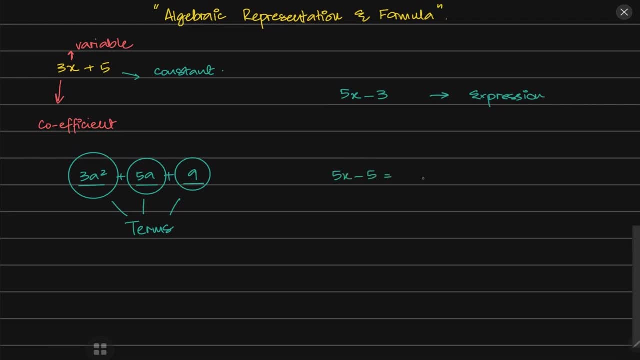 However, an equation is basically an expression, but equal to something, Maybe equal to four, maybe equal to zero, whatever. Okay, Now this is what your equation would be. Now, this is obviously the different types of equations that we're going to be doing: linear equations, or quadratic equations, and 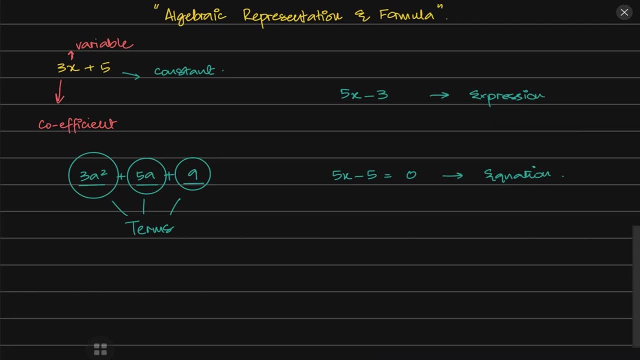 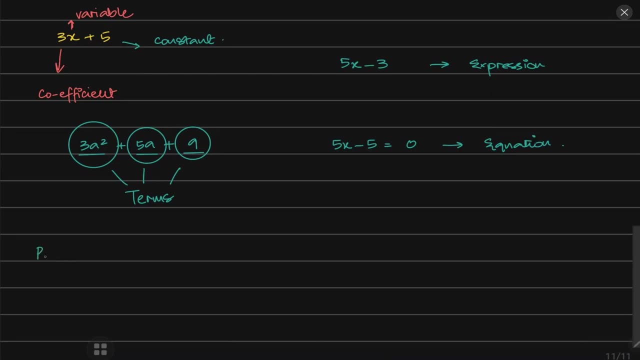 you know all these things, but those are different things altogether. There are different types of equations that you would see. Now we call these expressions or these equations as polynomials. Okay, So basically, all right, as they they. they basically consist of one or more terms, All. 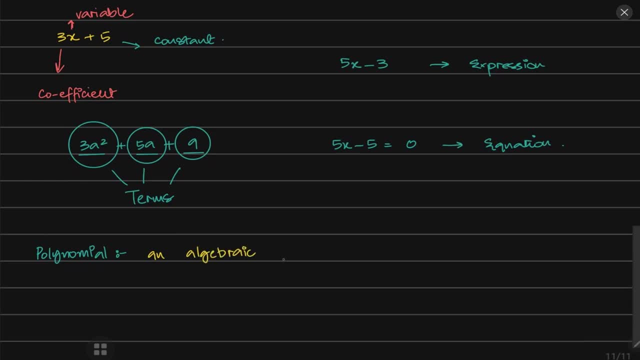 right. So polynomial is basically an algebraic. These are an algebraic expression which consists of one or more terms. Okay, Now, that's that. Now we have a question. Okay, So we have a couple of rules, basic, you know, basic algebra rules that we guys, I'm pretty sure you guys- 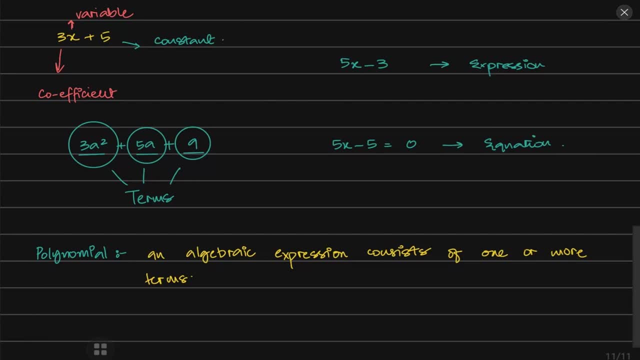 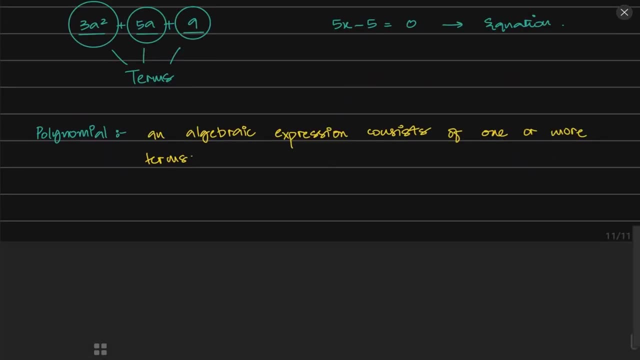 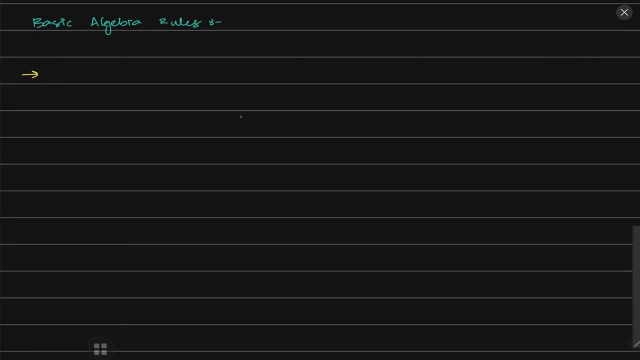 already know And there's a couple of basic algebraic equation algebraic equation rules that we're going to be doing. Okay, So, when we're talking about basic algebra rules, basic algebra rules- So the first one is that you're like terms can be combined or compressed into. 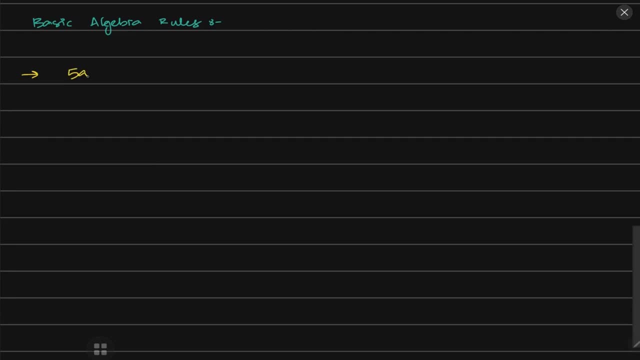 a single term. Now what do I mean by that? What I mean is that suppose I got five a squared plus two a plus seven, plus six a um plus three. let's say now you need to identify the like terms over here. In this case it's two a and six a. they're both the same things. 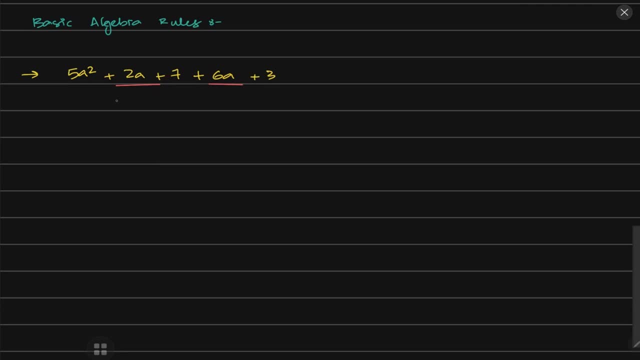 All right, The like terms are similar to each other, So what you can do is you can come to you know, combine them and write them as one. So plus two a, plus six a will give you a plus eight a, Similarly seven and three. over here There are light terms and you can just simply add: 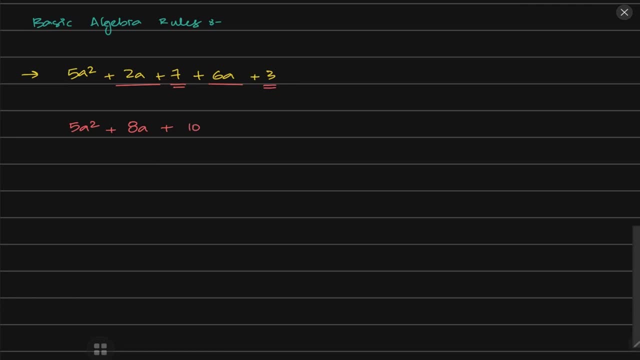 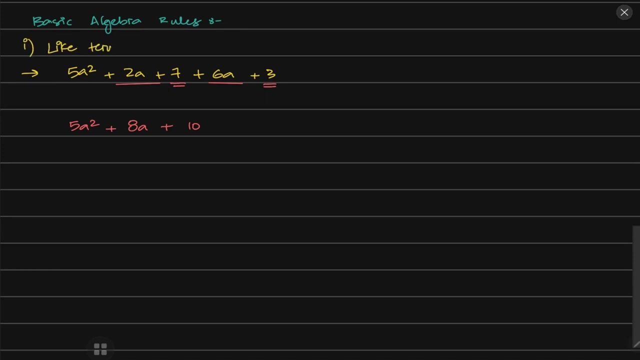 them or just do the mathematical operations whatever they're. whatever is there in the question, right? That's basically what the first law is, or the first rule is that you can combine like terms into a single term. Okay, So let's write that down Like terms. 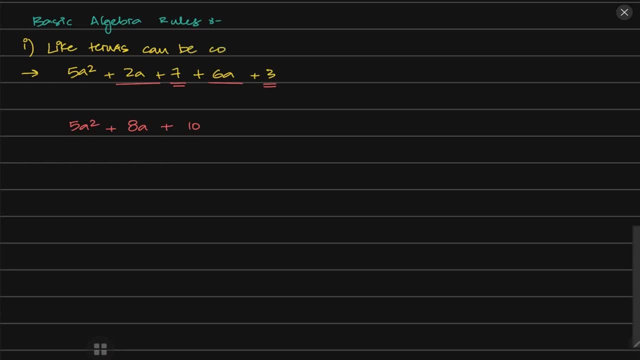 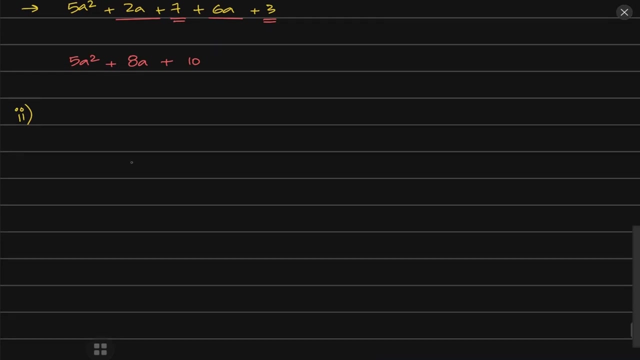 can be combined into a single term. okay, next up we have that whenever we're multiplying or dividing, right, the coefficients and the variables are basically multiplied or divided. okay, now, what do i mean by that? let's see, let's suppose i got 10 times 4, a times 2 a over 2 times 2 a over 2, right, in this case the coefficients. 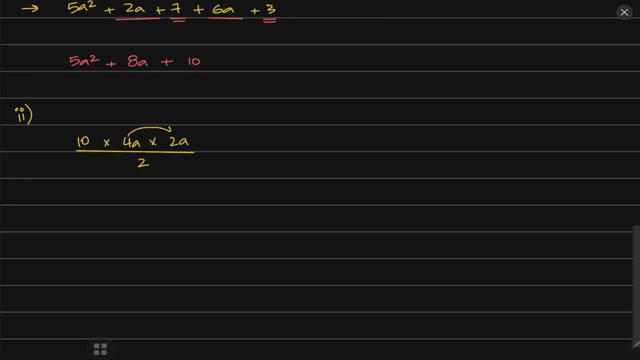 are multiplied together. so this 4 will be multiplied with 2, this 10 will be multiplied with 4. okay, and i'll get um 80 over 2 in terms of the coefficient. all right, but the variables are also multiplied with each other, all right. so when the variables will be multiplied in that case, obviously i have 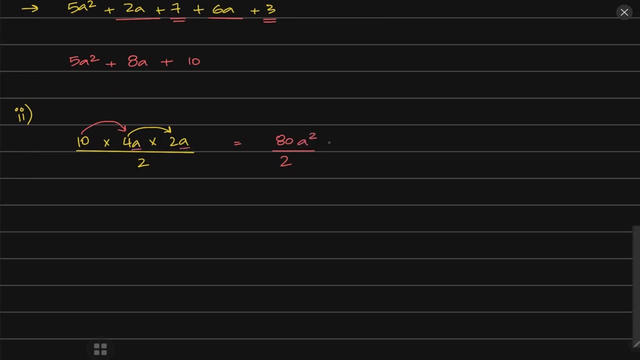 a and a over here. this will combine, multiply to a squared. that's what it's going to give me. all right. so you need to understand that when you're multiplying the coefficients and the variables, both of them will be multiplied with each other: multiplication or division, the variables and the coefficients. 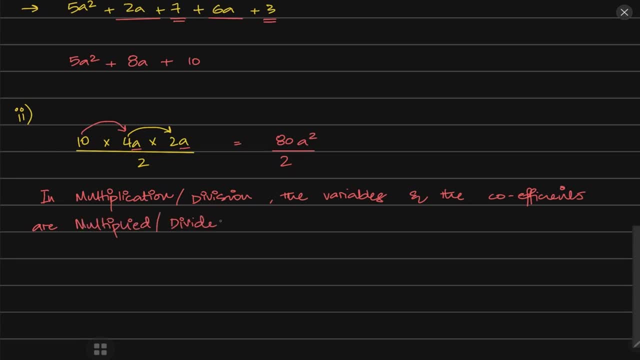 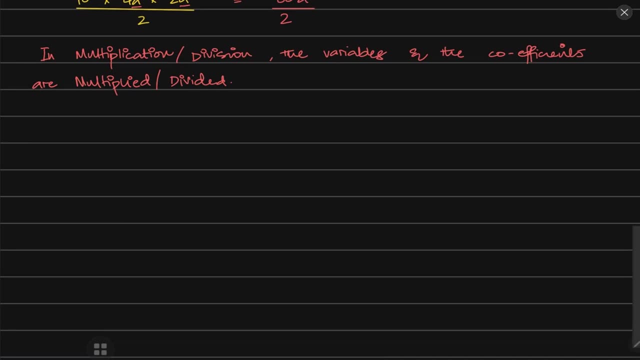 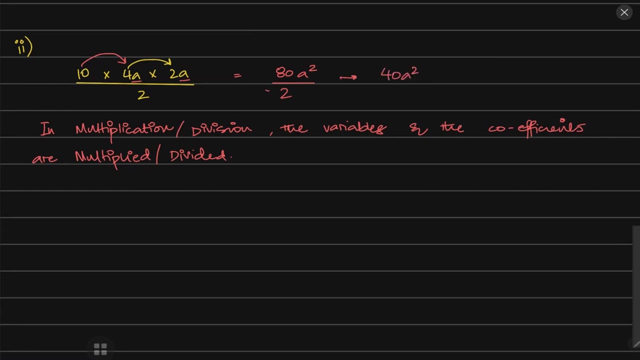 are both multiplied and divided. there you go right. and now, obviously, in the end, if you further simplify, you get 40 a squared, since obviously you have a, you have division happening over there. okay, let's see now. so, whenever you have an expression, all right, and the expression has obviously the 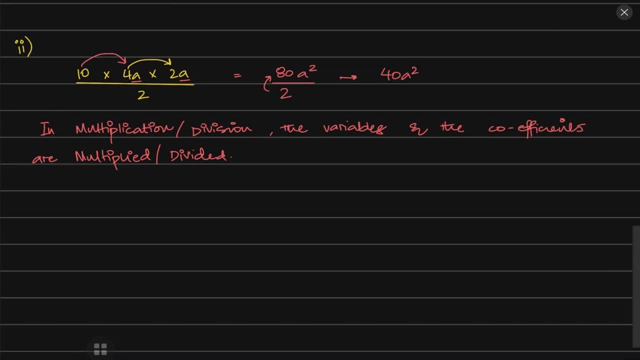 the expression has a number which is outside the bracket and it's technically supposed to be multiplied. what will happen is that each and every single term within the bracket it needs to be multiplied by that number. okay, now, what do i mean by that? let's suppose i have a situation. 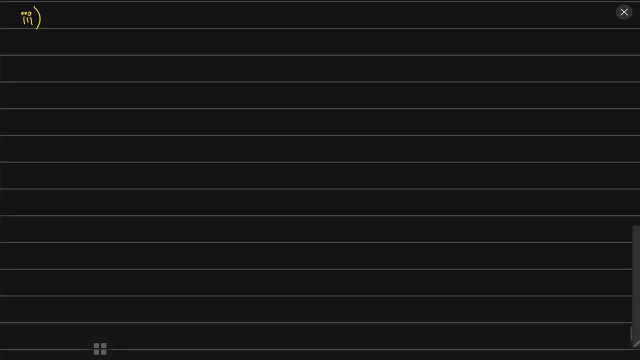 where i have a number which is outside the bracket and i have a number which is outside the bracket and i have a number which is outside the bracket and i have a number which is outside, i've got 5 times a squared plus 2a plus 4.. all right, so what i'm doing, i'll have to multiply. 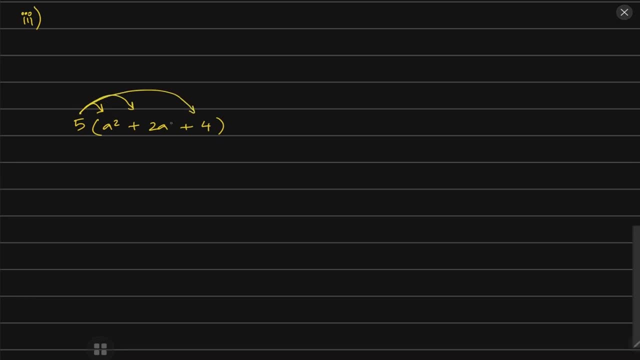 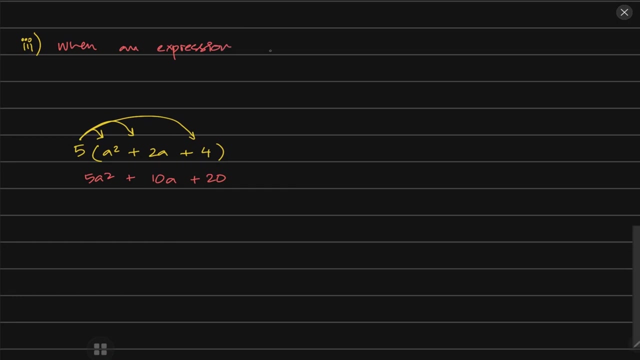 5 with every single term that's in the or within the bracket. so i end up with 5a squared plus 10a plus 20.. okay, so that's the third law, the third rule that you'll have. so when an expression in brackets, 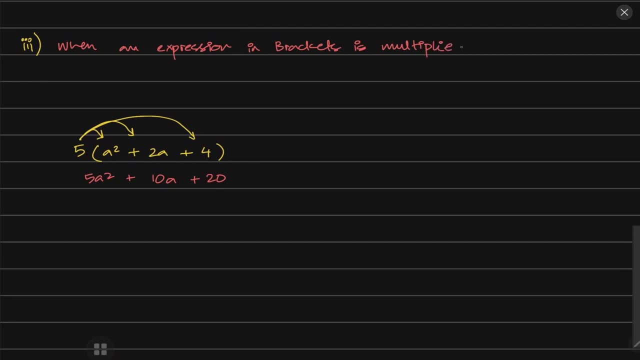 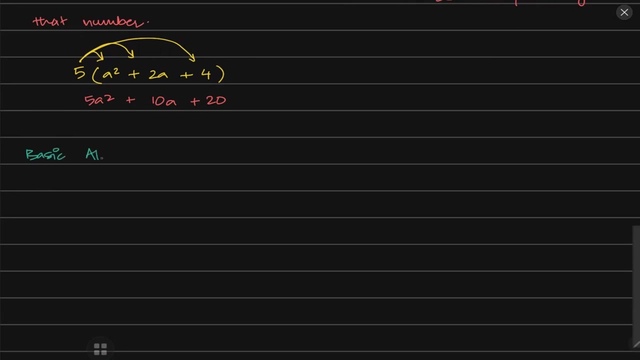 is multiplied by a number. each term within the brackets must be multiplied by that. okay now, i was talking about basic algebraic equation rules earlier on. um, i mean there's. i'm pretty sure you guys already know this. now let me write that down. so basic break. 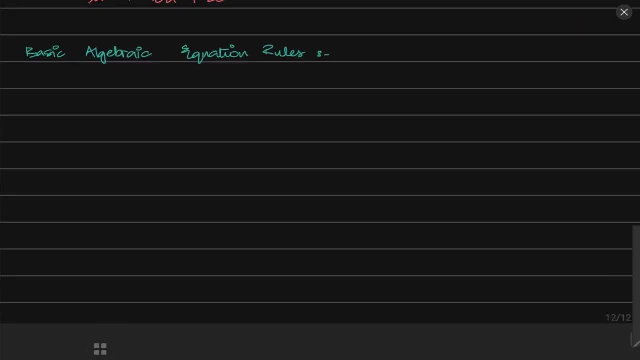 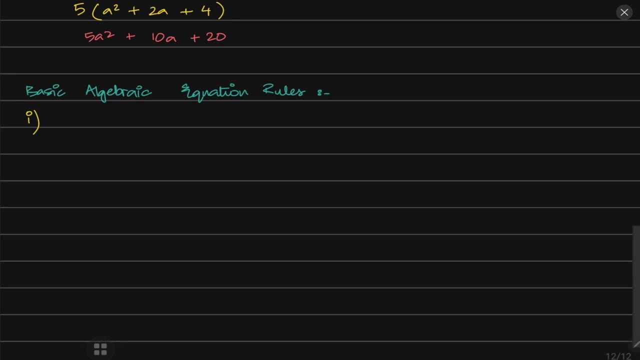 equation rules. let's see now. the first one would be that your numbers will be, or may be, added or subtracted from each side, if you're supposed to, you know, solve a certain equation or an expression, or whatever equation basically. but let's suppose i have x squared plus five equals to ten. right, what will happen is, it's not like i'm taking 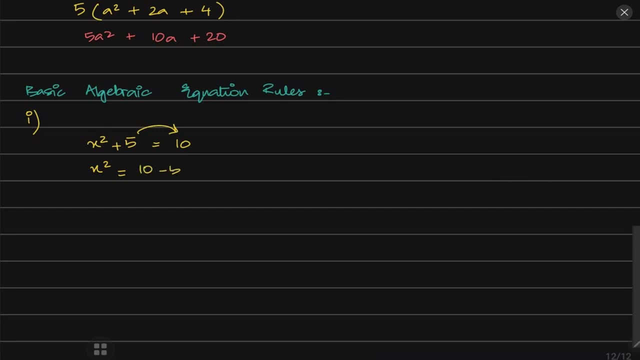 i'm gonna just you know, whenever i take it over there, this becomes ten minus five. that's not what actually is happening. what's happening is that you'd basically take. you know, it's the exact same thing. all you're doing is you're basically subtracting or adding the same thing from both. 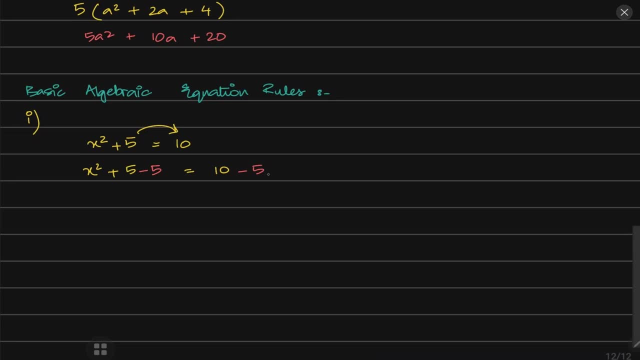 the sides. okay, so technically, this is what you get, this is what you, what we normally do, that's what our normal practice is, but on the backhand, this is basically what's happening. okay, so your, you can write down that equal numbers may be added or subtracted. 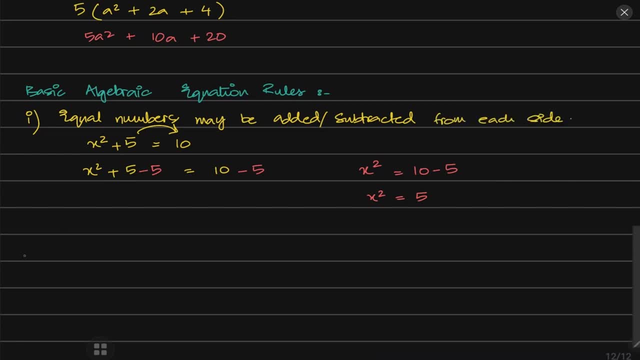 from each side. okay, now we got another pointer, same thing that you know. each side may be multiplied or divided by equal numbers, once again, except zero, because if you're dividing or multiplying with zero, then there's no point of doing it in the first place, right? so let's suppose i got um x minus seven. 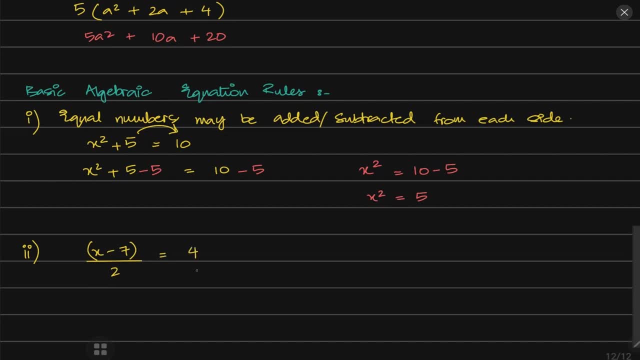 over two equals to four. okay, so what do we normally do? we just take this over here and you you get x minus 7 equals to 2 times 4. that's what we do, right, but that's not what's actually happening. what actually happens is that you multiply 2 on both the sides. 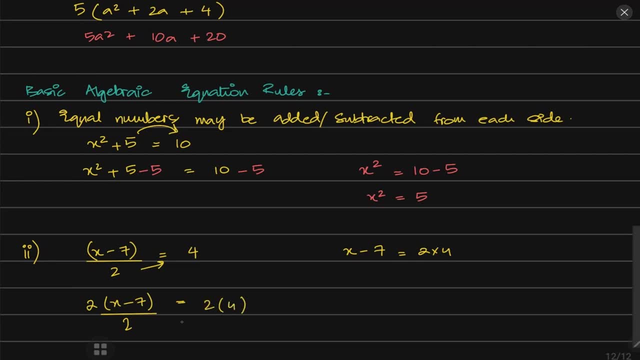 this with this 2, and this 2 is cancelled, and that's how you get x minus 7 equals to 2 times 4, okay, so another point that you can write that each side may be multiplied or divided by equal numbers. okay, except zero, obviously. 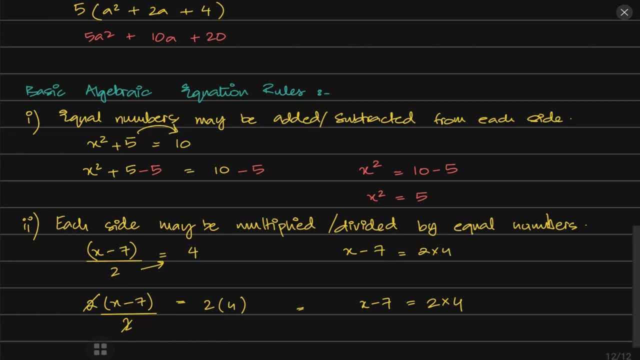 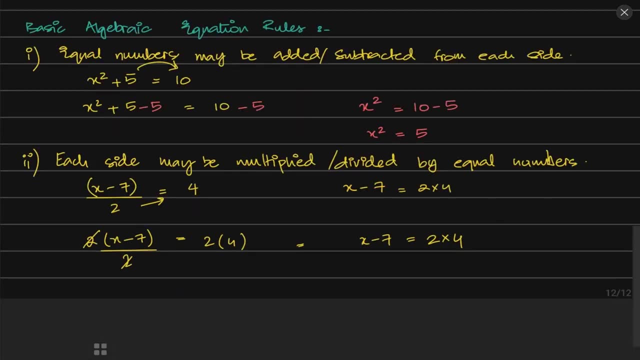 okay now, uh, that's basically. uh, that's basically it. that's about the, the. you know the basics of algebra. now we're going to start off with algebraic manipulation. okay, this is the real deal. this is something that you guys will probably be doing more. okay, but once again, 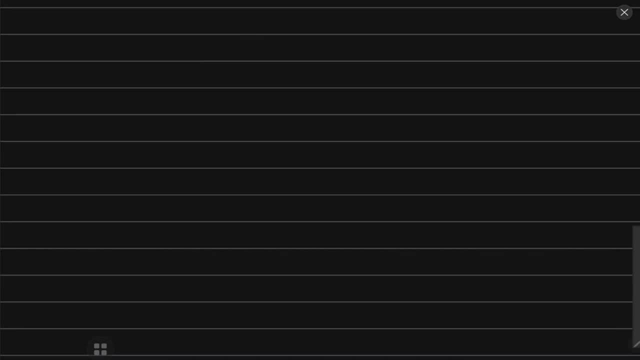 it was important first to understand how things were done on the basic level, first to talk about this. okay now. okay now, algebraic manipulation. this is basically how you play with algebra in your course. okay, now, the examiner might test you in a couple of ways. all right, the first thing. 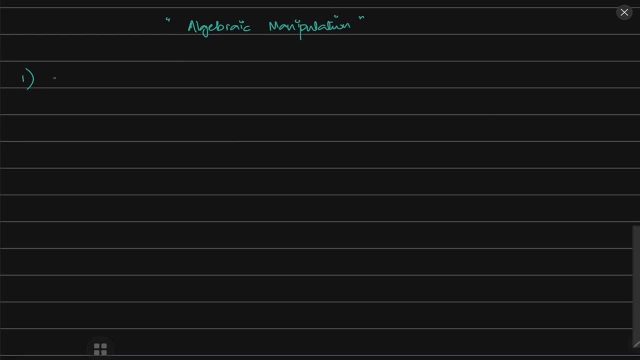 that the examiner might give you is to they might ask you to change the subject of your um, of the question, right, right. so i'm sure if you've done uh, if you've opened the book previously, if you've ever tried out these questions, you will have a question where the examiner gives you an, uh, an equation. let's suppose you 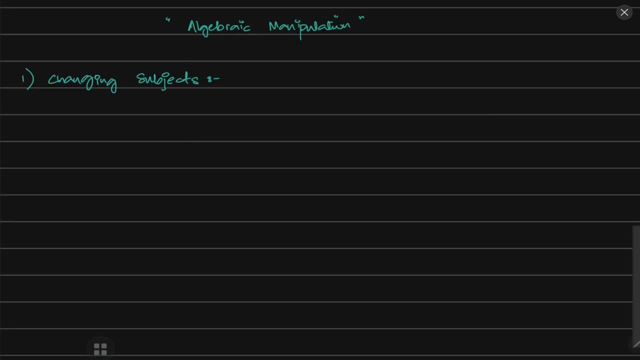 have an expression or, sorry, you have an equation that goes like: y equals 2, x plus 5 over x. well, let's call this z, actually, okay, and now they're asking you to this square two, but we don't get that line, it's all. but it's called a. 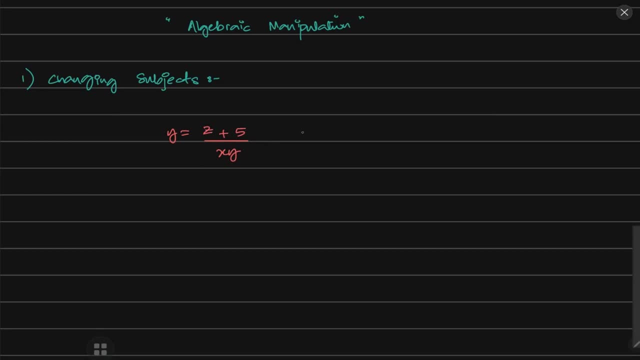 z x squared. county f minus x times x squared. if there is no�, so taken you to x and y equals. this can create the condition right now. the set what's going to space of x and X and y and Y is is actually pretty, pretty, pretty correct. 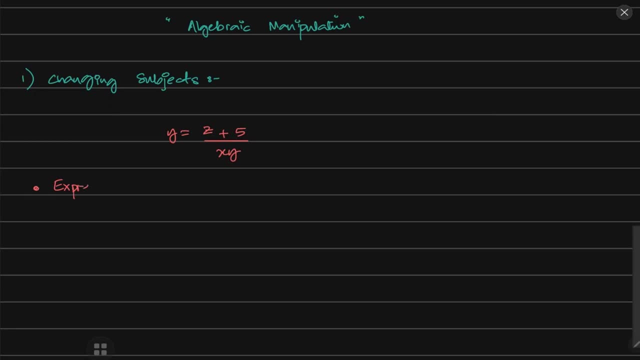 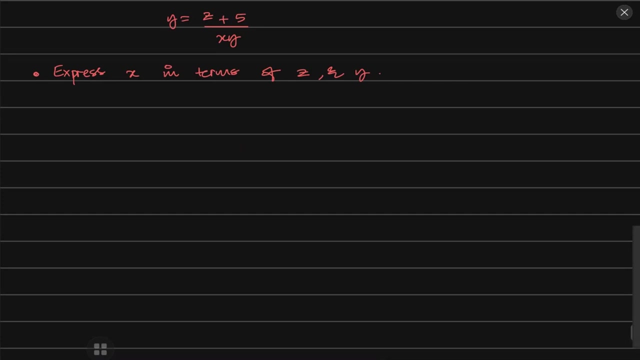 this is what the question says. question goes: they express x in terms of z and y. okay, now, in this case, what you're supposed to do is you're supposed to rearrange. okay, you're gonna rearrange the entire thing to make x your subject right now. what do you do? you? 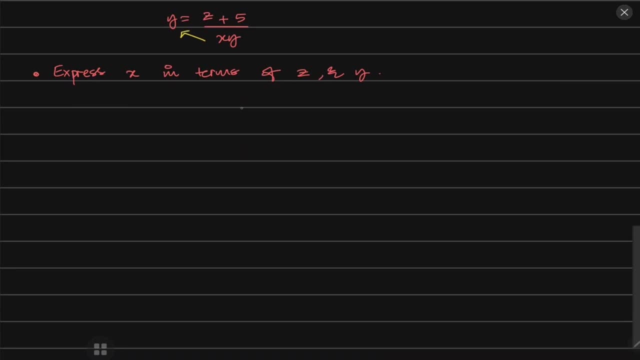 basically take, you know, you multiply on both sides with x- y, or you take it on the other side. in other words, this will be x- y squared equals to z plus five. right, and that's how you get x equals to z plus five over y squared. okay, fair enough, so, um yeah, so the second thing. 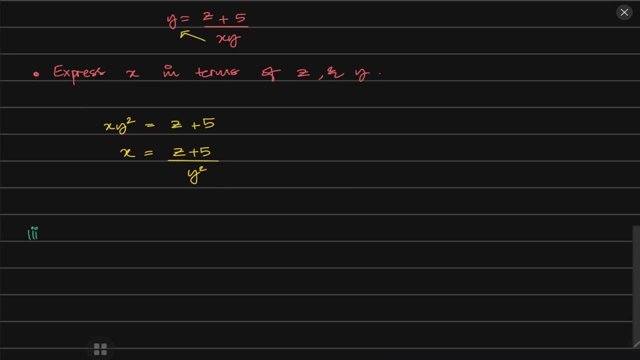 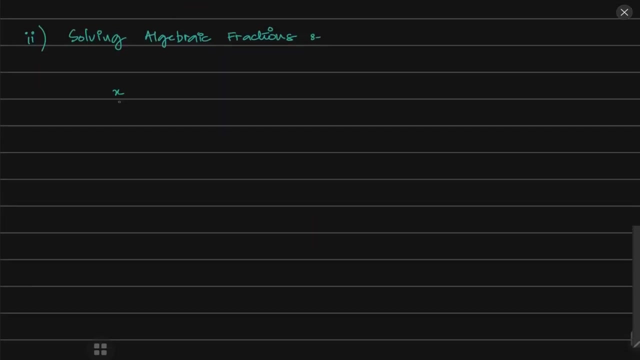 that the examiner might ask you is when you are. they would want you to solve algebraic fractions. solve algebraic fractions. okay. now, in this case, let's suppose i got a question that looks like this: um one, four equals two. let's say x. what you do is you'll have to take the lcm. 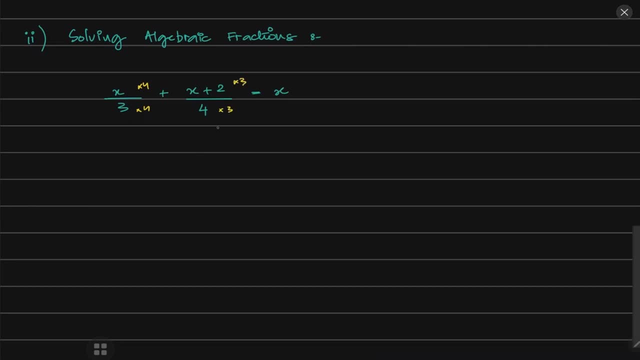 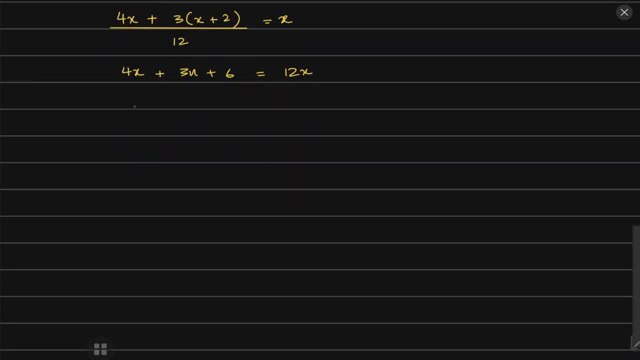 in this case, and solve accordingly. all right, so you get four x plus three times x plus two over 12 equals two x. then you'd have four x plus three x plus um six. this 12 is going to go over there, it's going to be 12 x. let's say you get 7 x.